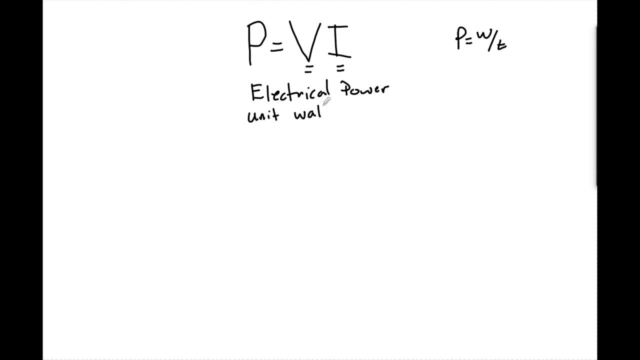 so the unit for this is also going to be watts. So essentially, what we have to do is we have to use Ohm's law, And remember that Ohm's law is equal to V, I, R, where V is a potential difference. 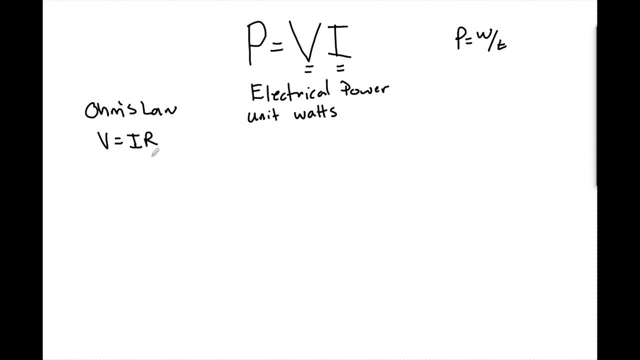 I is the current and R is the resistance. Now this can be applied at the battery for total power, Or this can be applied at each and every resistor. So, essentially, what I want to see is what happens when we are not given P, V and I. Well, one thing we can do is we could say that V equals I, R. 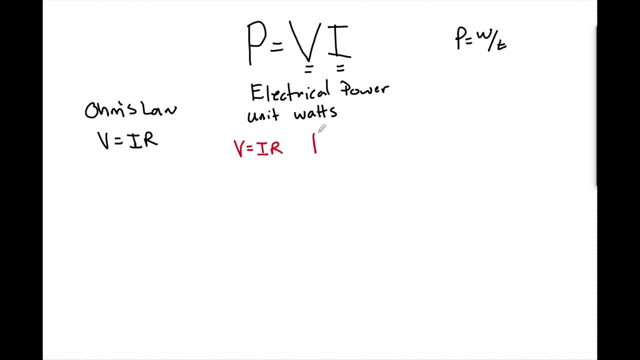 right. So if I look at this formula now, I could say that P equals that substitution for V, which is really I R times the original i that I had in the formula. So now we have a variation of the power formula, which is just P. 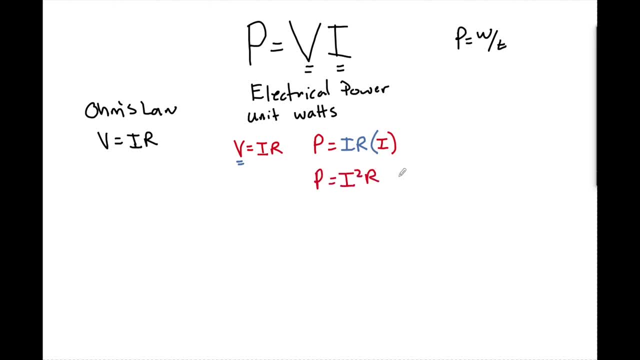 equals i squared R. And this is when we don't have voltage potential difference. OK, So this is how we are going to be able to solve for P without V. Now the same can be done because we know that I is equal to V over R. So if I look at that power formula, I can now. 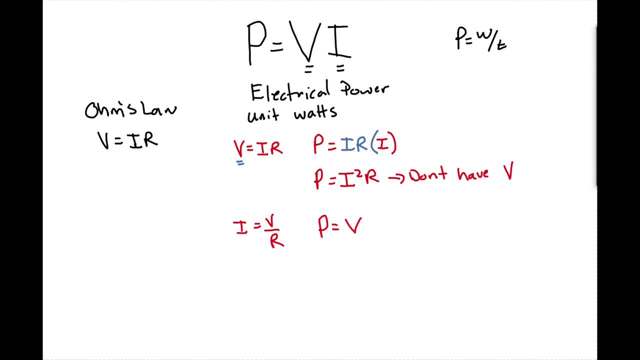 say, P equals V times the substitution for I, which is V over R, to now get a new power formula that's equal to P equals V squared over R. So this is how we are going to solve for power when we don't have current. So we can see an example of this. 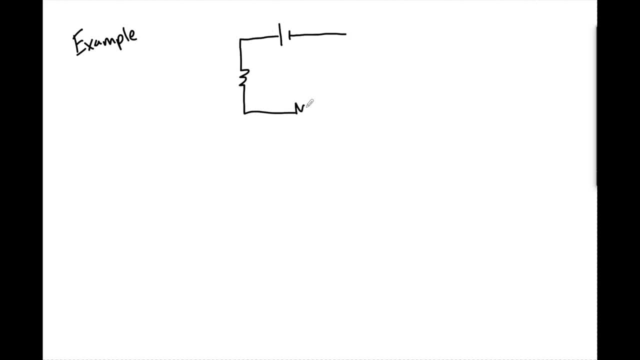 Let's say I have a series circuit and it has three resistors in it and I know at this resistor right here, R is equal to four ohms and the current here is equal to two amps and I want to know what is the power at this resistor? Now we would look traditionally and we would say P equals VI. that's on our 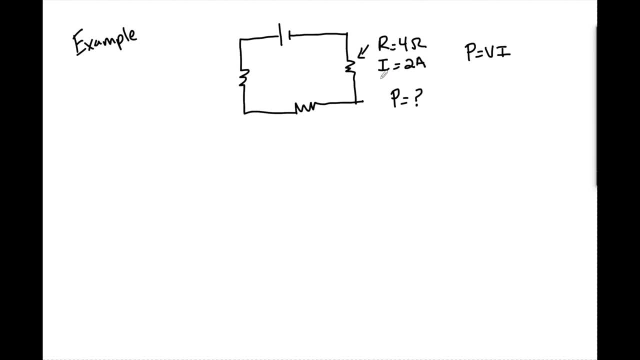 reference table. but we don't know what V is in this case. So we have to go and say: what do we know? V equals Well, P equals. V equals IR. from Ohm's law times, the I. So now we are caught in a situation where we just have 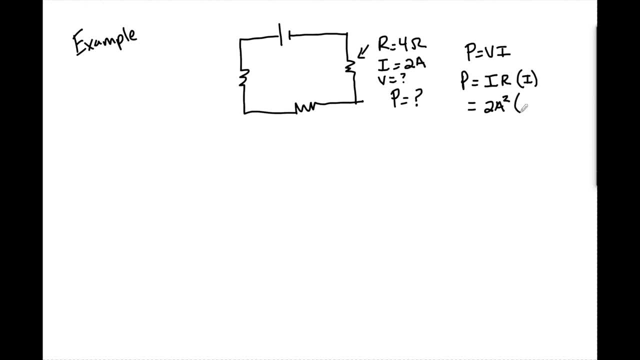 two amps squared times four and that's going to be equal to 16 watts. But if we look at, say, R1 over here and we know that the potential difference here is equal to three ohms, Equal to 12 volts, and the resistance there is equal to three ohms, 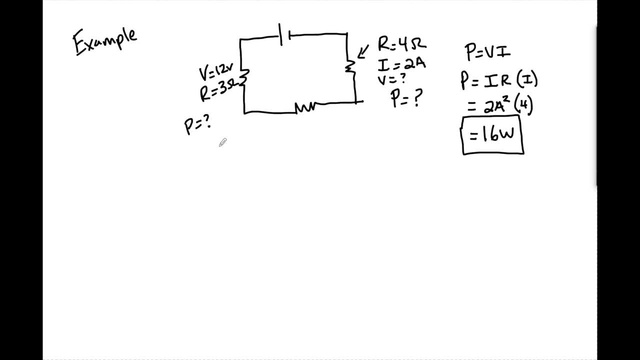 I can now find the power here as well. So we know that P equals V times I, but in this case I don't have I, So now we have V times V over R, which is a substitution for I, So we have 12 times. 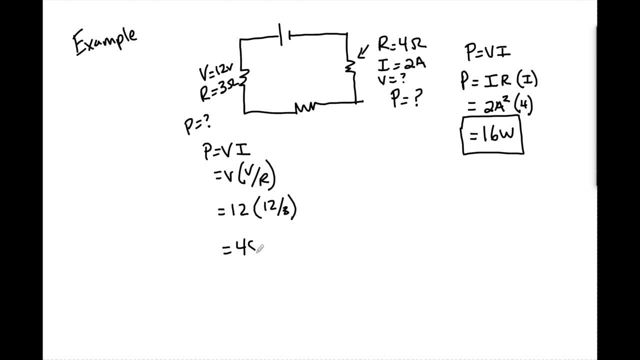 12 over three, which is going to be equal to four ohms. So that's going to be equal to 148 watts. Alright, that's pretty much how we are going to use the electrical power formula and how we substitute in Ohm's law.